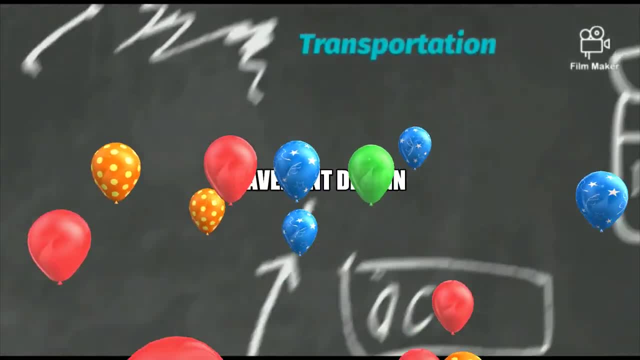 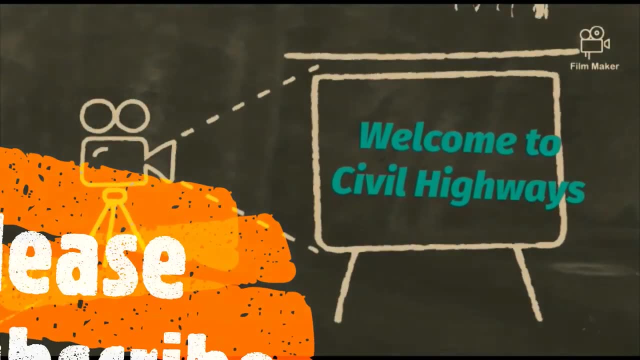 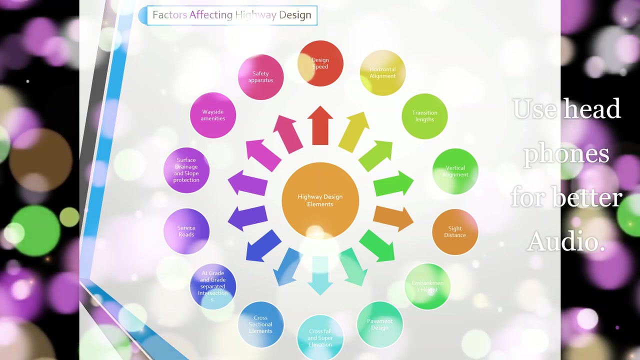 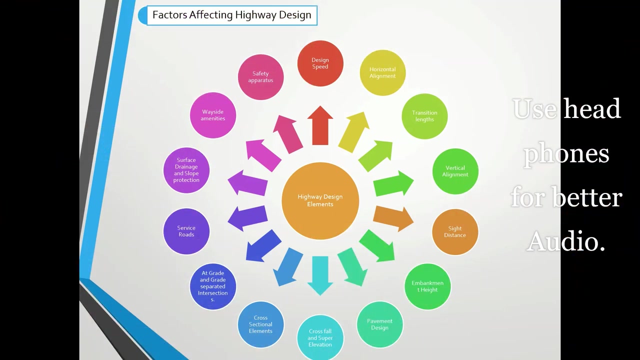 Hi, friends, in this video I am going to explain the things related to the factors affecting the highway design. Okay, so can you see the image? Okay, I am going to explain the things one by one. Okay, what are the important factors while doing the highway design? Okay, how are we going to? 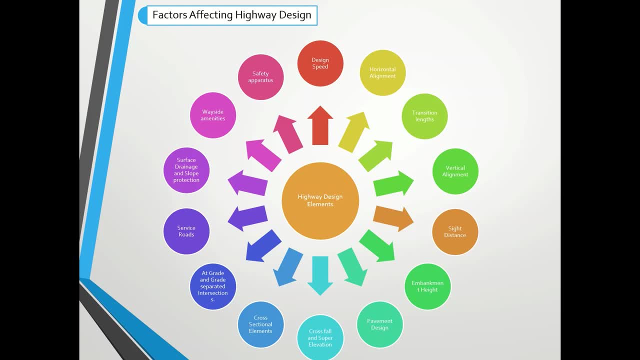 affect Means. what are the considerations we have to take while designing particular type of design elements? Okay, these are highway design elements. Okay, these are just a few elements only, but these are, means, very important highway design elements. Okay, if you complete this, almost. 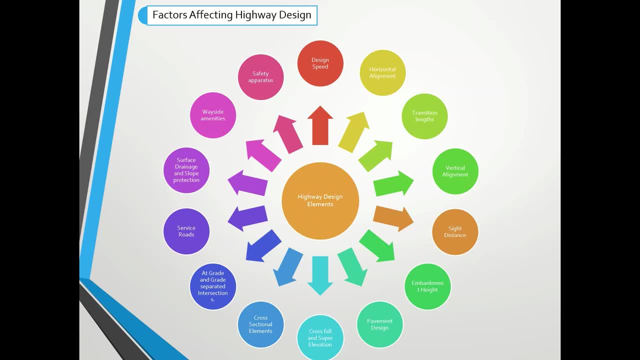 highway design parties, 90% gets completed, Okay, so let us go one by one. So first one is design speed, Okay. then horizontal alignment after the transition length criteria, then vertical alignment after that side distance, then embankment height, then pavement design, very, very very. 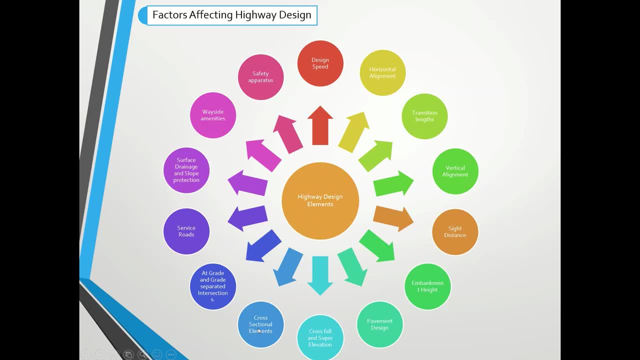 important. then cross fall and super elevation, After that cross sectional elements, nothing but paved shoulder verge, carriageway, all those things will come. And then at grade and grade separated sections, very, very important. highway design element- Okay, and then service road also. 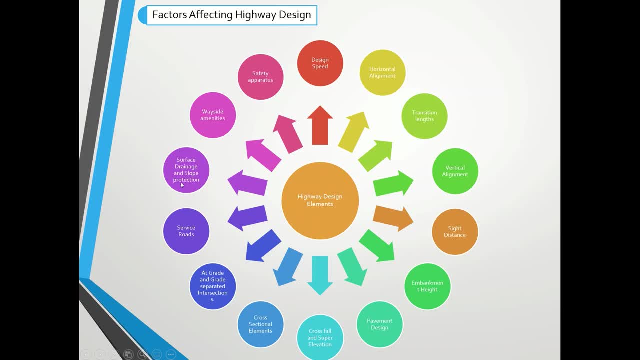 one of the part. Okay, and then surface drainages means normal RCC drain, earthen drain, okay. pipe drains, different type of drains, Okay, that also a part of highway design element then, where side amenities, nothing but toll plaza track lay-by like that. then safety apparatus. 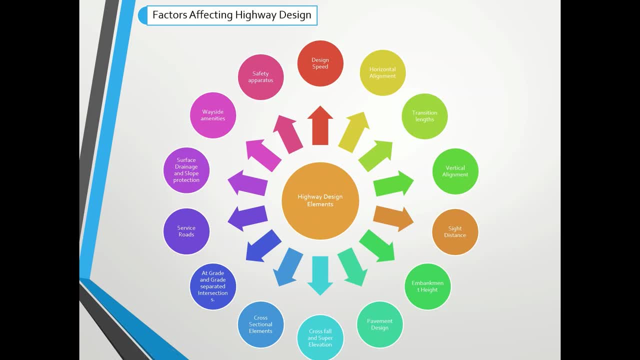 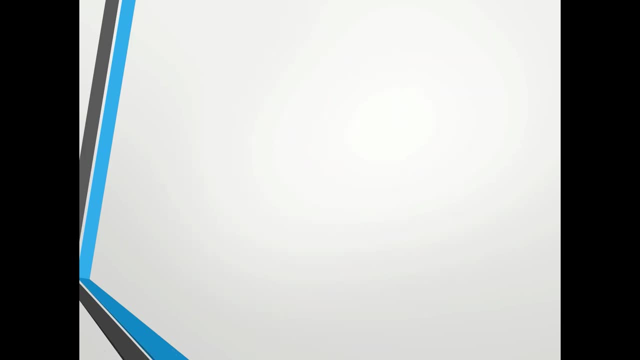 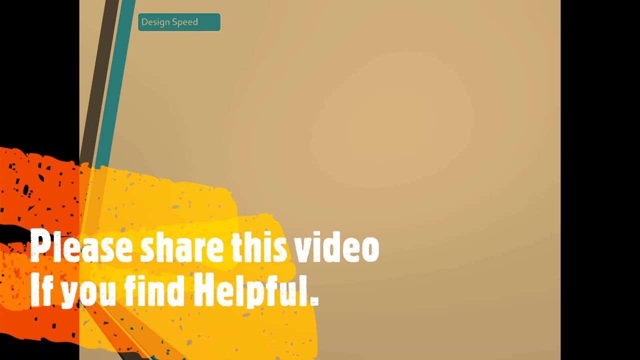 Normal, the crash barrier, the means vehicle restraint systems, nothing but Okay. so one by one, I will go. Let us start. Guys, please subscribe my channel and encourage me to do more videos. Okay, so next. first one design speed. So while doing any type of road, first 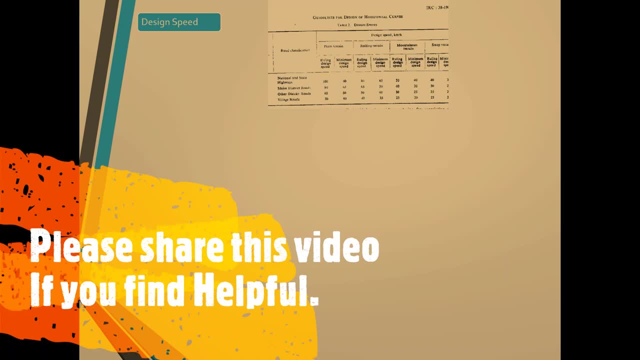 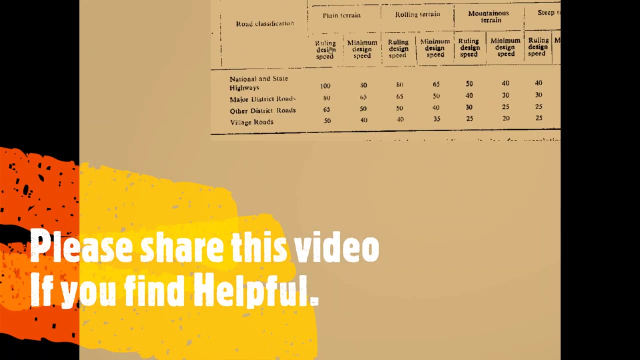 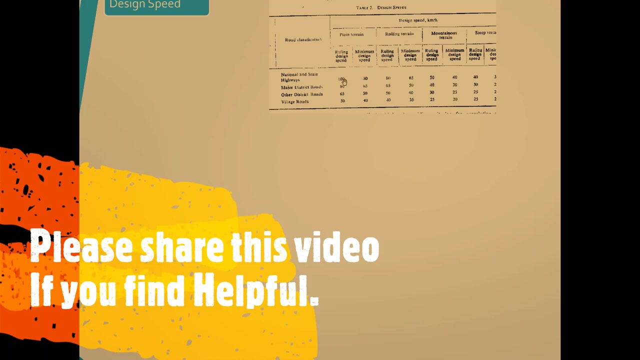 priority will be deciding the design speed. So there are codes and standards and you can refer it. for National Highway, Yes, it is 100, but in plain terrain, based on the terrain also, it will differ. So according to the speed you have to start the work. Okay, so that's the important criteria. So, based on the terrain, 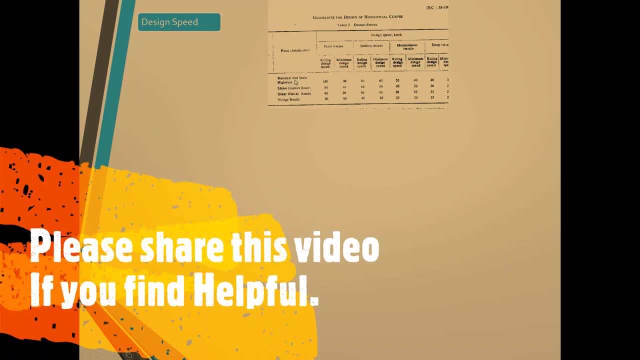 you have to decide the speed and type of road, also If it is State Highway 100 or National Highway 100. Nowadays, expressways are designing with respect to the 150 or 120 speed, especially greenfield highways. Okay, It will be less means 100 might might be there, Okay, so if it is greenfield way they are going with. 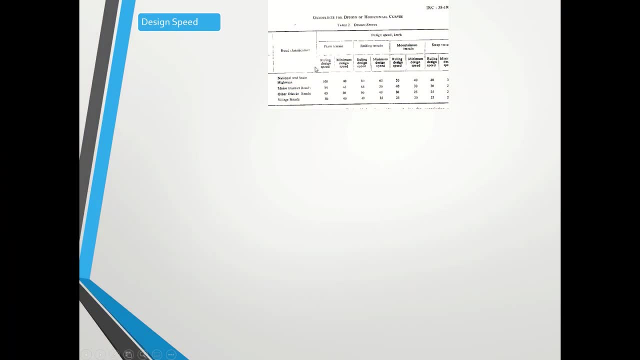 a higher speed only. Okay. so design speed is very, very important. Highway design element: Okay. so next, horizontal alignment: Okay, horizontal alignment First one is minimum horizontal curve radius. Okay, this is entirely dependent on the design speed. If you are following 100 speed, what? 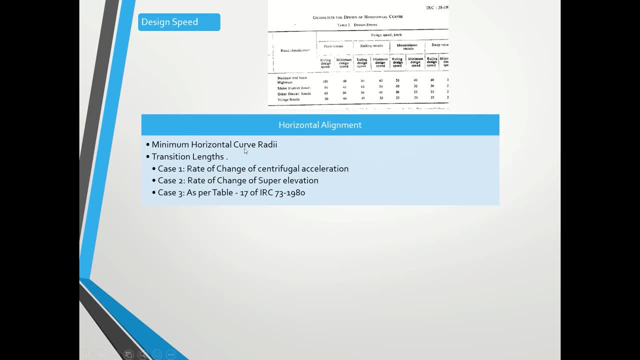 will be the minimum curve radius we need to provide. It should be around 360.. Nowadays it is increased to the means the standards increases to 400 meter. Okay for four lane road or whatever. Okay, if 100 speed minimum curve radius should be 400. Okay so. 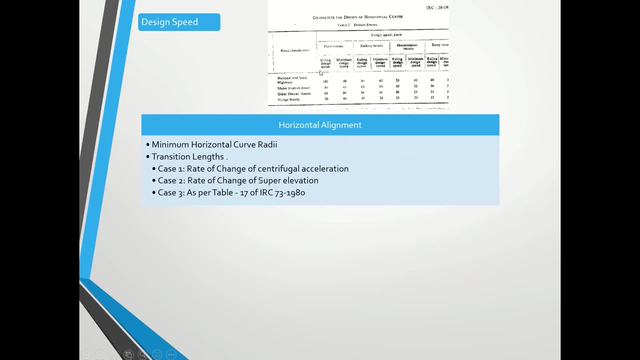 that they have given in a higher age manual man IRC SP 84 they have given, So you can refer it. So first important criteria in our general element is curve radius after the transition length. transition length means How you are going to provide. there are three cases. rate of change of centrifugal acceleration: vq by 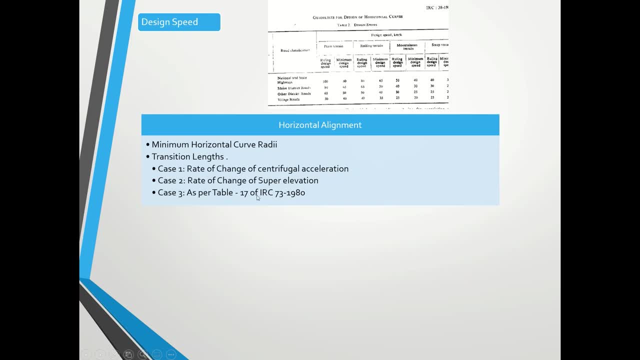 CR and then EB by two under, as per table of 17 of IRC 73.. Okay, so these are the three criterias. we need to take it. Okay. Accordingly, you have to design and provide the transition length. Okay, So then can you see the? 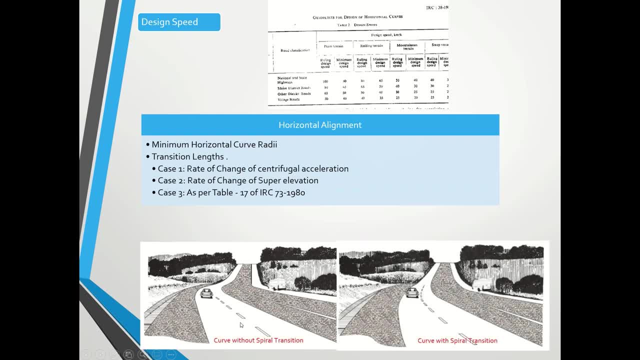 image: Okay, See, curve without spiral transition. Can you see? And then curve with spiral transition, how smooth it is Okay. And main transition provision is for the to contract the super elevation Okay, to enter vehicle smoothly, Okay. So that's why we need to provide the 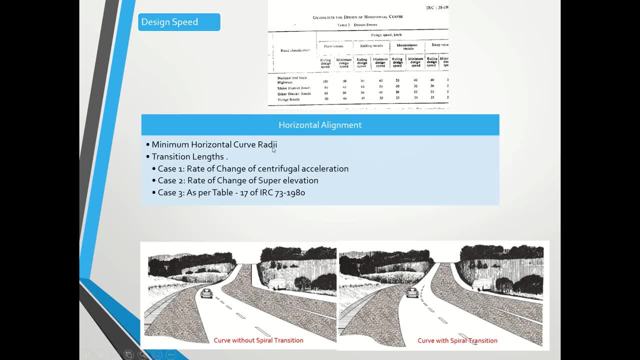 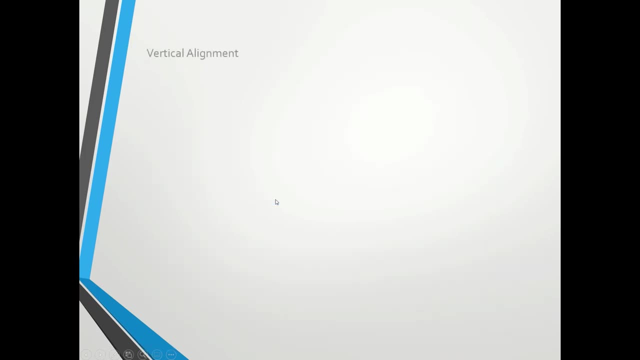 transition length. So it is very, very important. horizontal means design element, highway design element: transition length. So you must check with the standards and before submitting to the client. So transition lengths are very important, Okay, And then vertical alignment, Vertical alignment, Very, very important thing is: 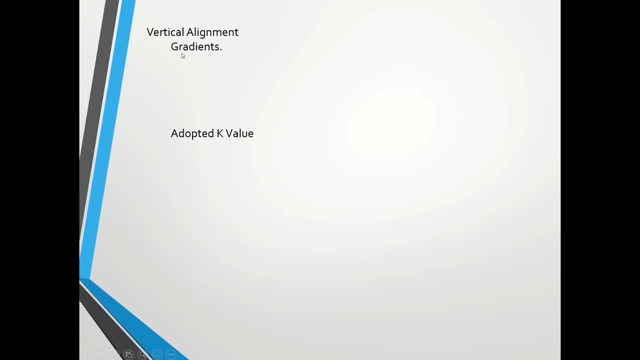 gradient. Gradient is the main factor affect the power of the vehicle means. So if higher gradient power required is more under he, the vehicle can't achieve the desired speed. nothing but design speed. Okay, there are standard can see for particular hundred speed. this ruling gradient is 2.5%. 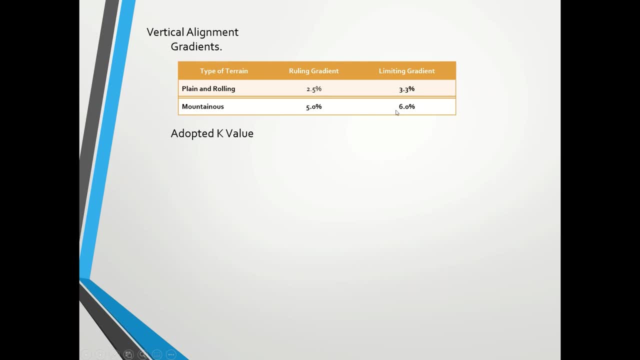 Limiting Is 3.3%, and then mountain is 5% and 6%. Okay, So that is the. these are values from the code on day I copied it. Okay, Then, after gradient, the very, very important thing is K value. Okay, So K value is nothing but a relation of the length of curve and 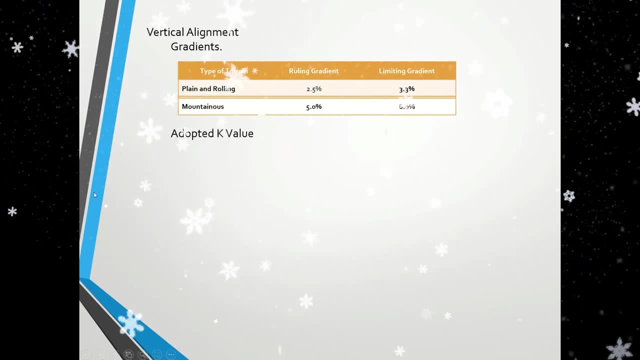 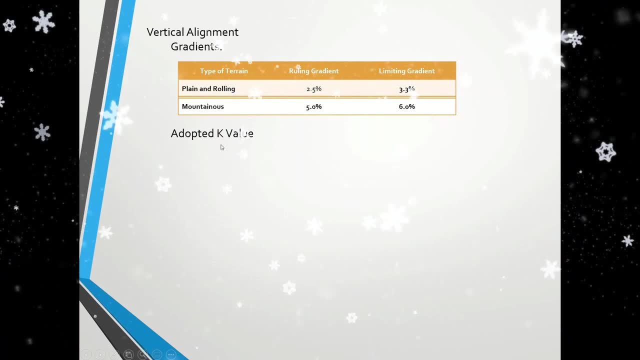 sight distance. Okay, Indirectly. if K value gets satisfied, automatically, sight distance will be achieved And the length of curve criteria will also be achieved. K is nothing but length of curve by the algebraic difference of the gradient Okay, L by a Okay, K equal to L by a Okay. So these are some. 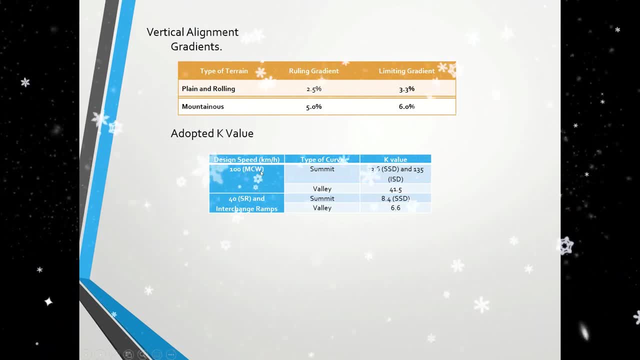 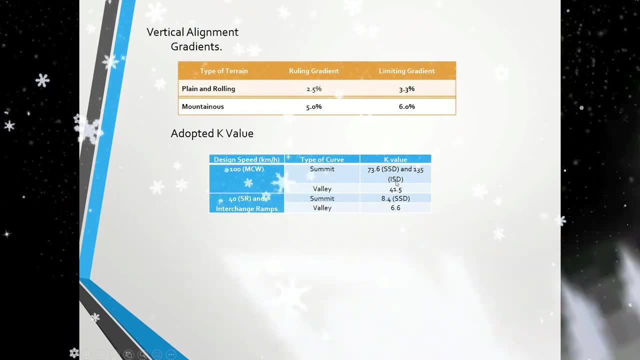 standard values for design speed 100. main carriageway For summit curve is around 73.6 and 135 is ISD For ISD. ultimately that what to say value will get increased. So that's why we have for valley curve it is 41.6.. 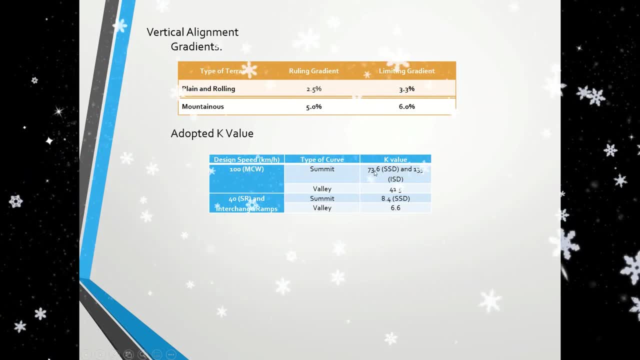 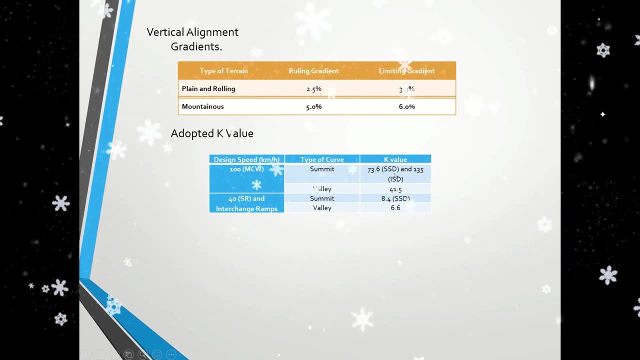 so while doing 100 speed the k values must be in this range. it should not be less than 41.5 and it should not be less than 73.65. okay, so if it is less than it you are deviating the manual. so be careful while doing the k value. vertical alignment, then this is for service road, so values. 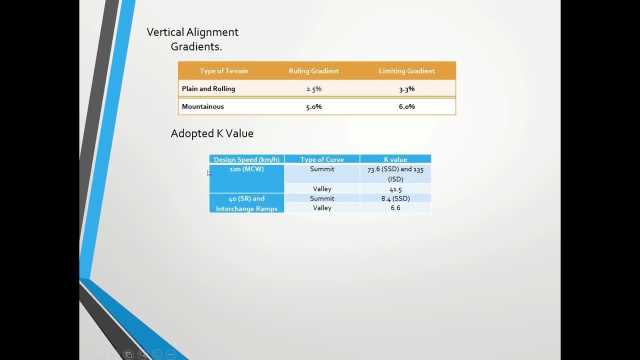 are different because speed is reduced. okay, this k values will get from the l equal to n square by 4.4 and 9.6. some values are there in irc, sp 23. okay, from the that only we used to get. okay. so then side distance. so side distance is directly relation with the k value. no need to worry about. 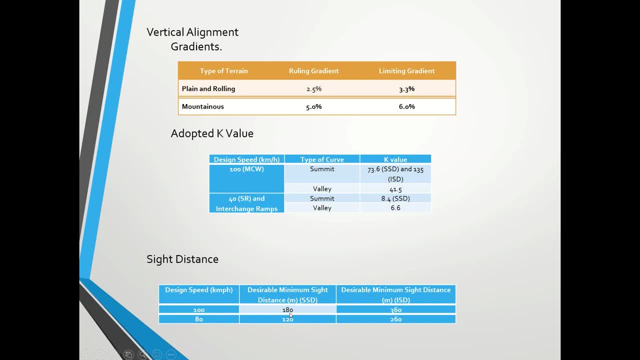 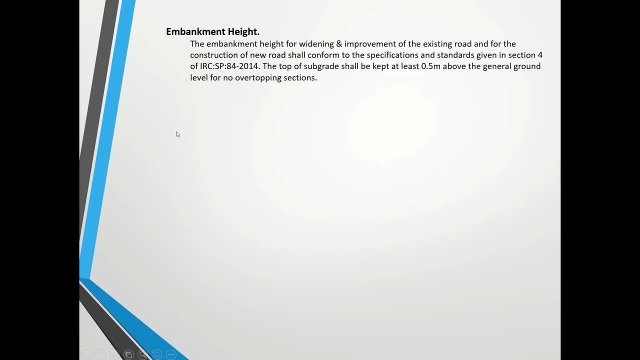 that no need to remember also, but if you remember it will be better means better. okay, that's it. okay, these are for the 180 speed. okay, and then i'm back you. So very, very important criteria while doing the vertical alignment. yeah, you know the maximum grade. 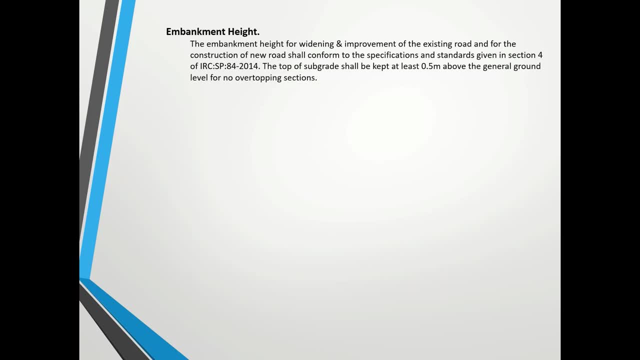 and minimum grade values and k values. all things you know. but how to proceed means how much height height we need to rise based on the existing profile. so that can be. that can be done with the criteria in irc sp 84. they have given one condition, so embankment, height of widening or improvement of 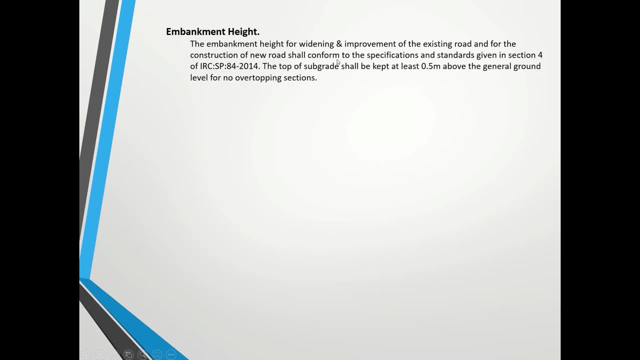 the existing road and for the construction of New Road shall confirm to the specifications and standards given in the section 4 what they have given. the top of subgrade shall be kept at least 0.5 meter above the general ground level for no overtapping sections- overtopping. 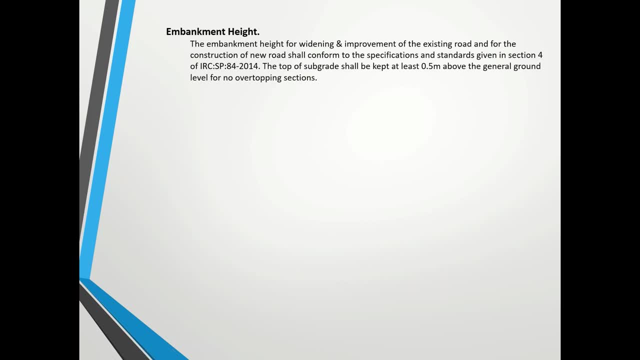 sections means nothing but flood effected areas. okay, so that is the one. so embankment height criteria is very, very important. you can refer this section for. okay, that main thing is the at least 0.5 meter above the general ground level. okay, top of subgrade, not bottom of subgrade. 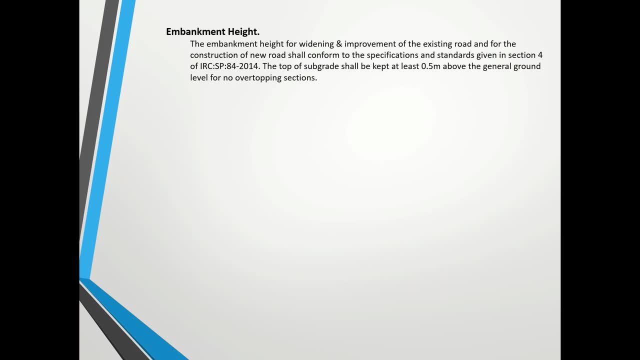 okay, 0.5, and then 0.5 meter subgrade, then about whatever the criteria means: uh means gsb, always will come, at least means approximately 1 to 1.5 meter height we need to raise okay to from the existing ground level. okay, so that is the important criteria: embankment height, and then 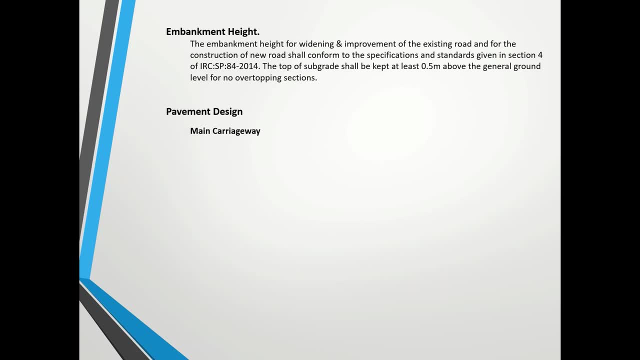 one of the important thing: payment design. payment design we have to do for main carriageway and service road. both we have to do separately because in service road no need to provide that much higher thicknesses because msa will be less. normally we used to consider 10 msa like that. 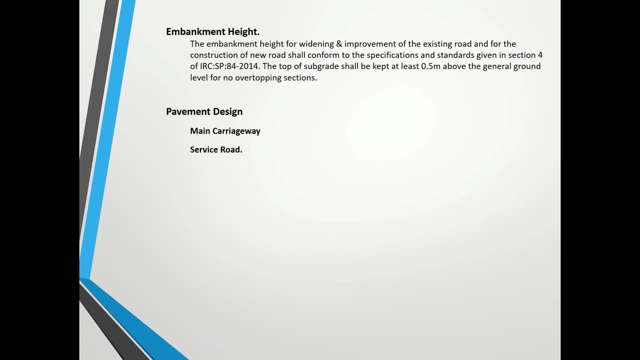 for service roads, but main carriageway we have to calculate based on the traffic data. and one more thing: toll plus also we need to calculate the. we need to evaluate payment design. okay, that also one thing, i haven't mentioned it, but payment design you have to. 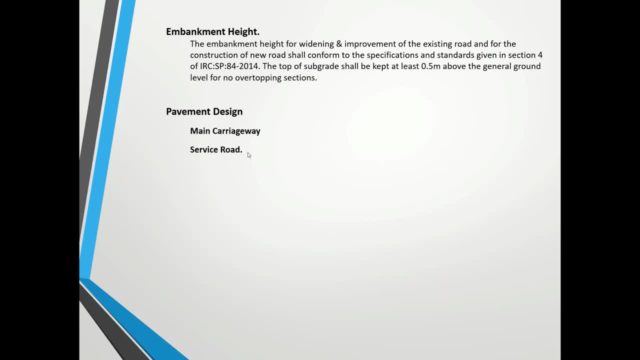 do for these three sections, okay, separately. okay, based on the different msa. okay, and i have prepared for you, uh, other section for the disassembly or for all the letzten section. you can give about which detail ako? thank you very, dw, okay. okay, guys, so from here you can use this. 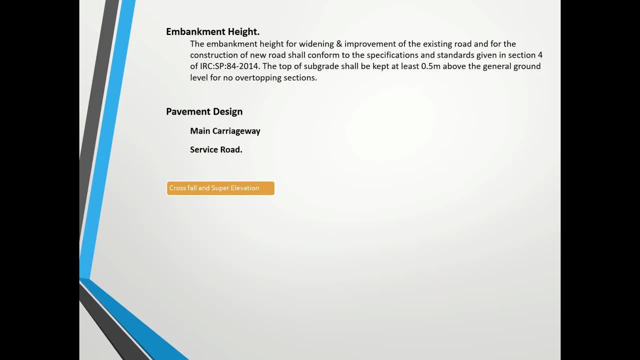 function. okay, this is the second section. okay, in this section. okay, you need the detail of the head and manufacture of four units. okay, two units. okay, right, for evaluation, be 2.5 percent for rigid, two percent. okay, for earthen shoulder, it always 0.5 percent greater. 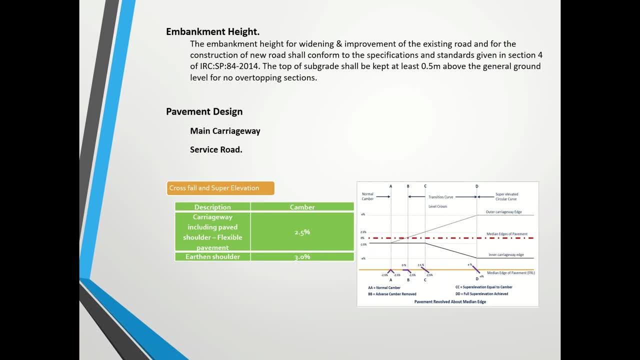 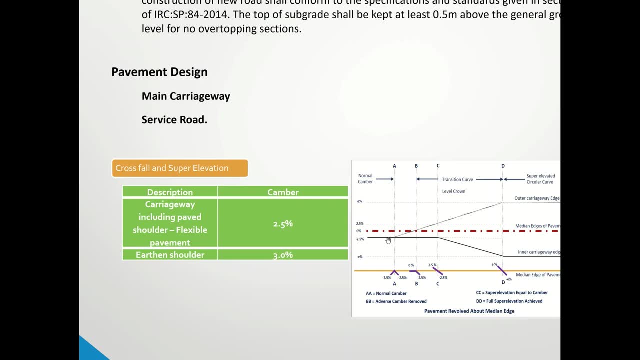 than the camber. okay, whatever we are providing. and then super elevation: very, very important topic. okay, so while applying any means, mnc companies, you must have a look over the super elevation nodes and thing. you must be aware, okay, how we are going to apply. okay, so can you see here? 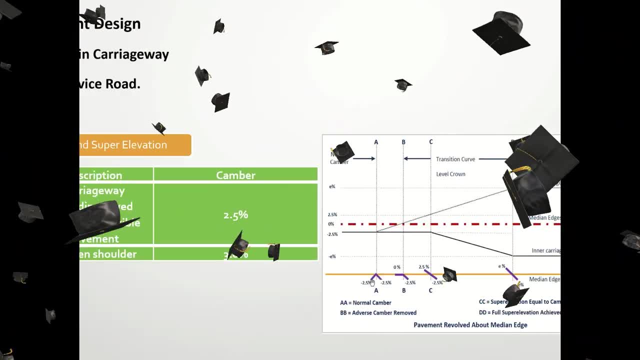 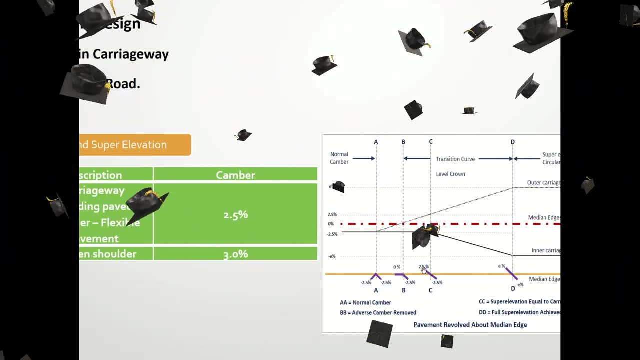 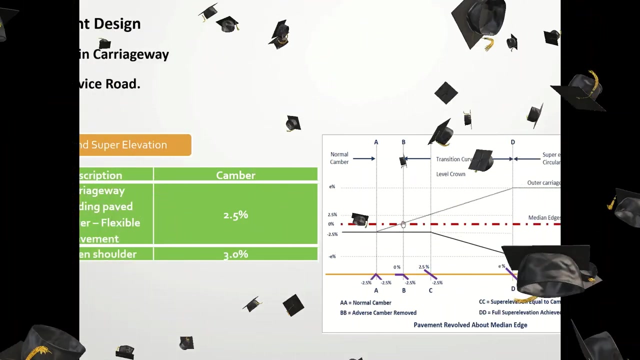 can you see this normal camber and then outer edge raised to zero percent, then outer edge size to 2.5 percent, like this? okay, then it will achieve to the total okay percent, whatever. okay, see a transition. it should be zero. okay, can you see this rotation outer carriage after that, at curve only we need to achieve the. 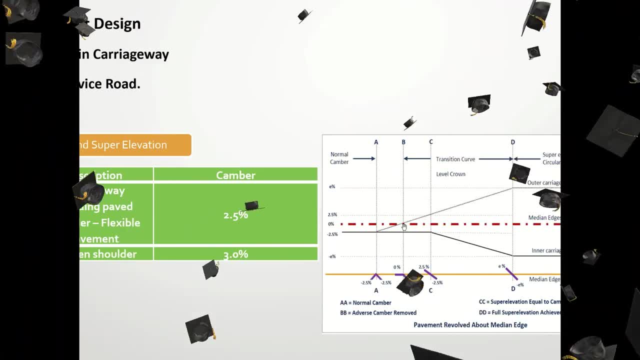 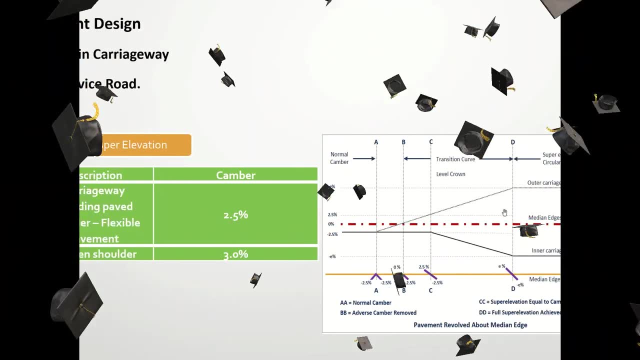 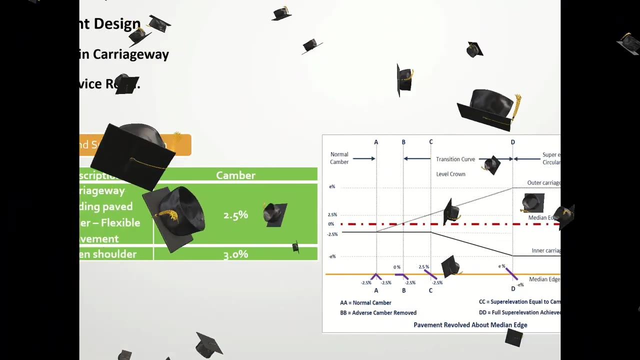 entire entire super relation value from zero to e value and then from normal camber to zero. okay, so that is, we need to means we have to understand the how the super elevation is applied and you have to check the cross sections while doing the design after applying any super elevation. 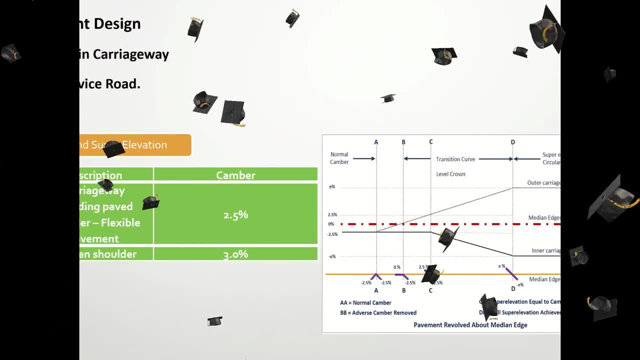 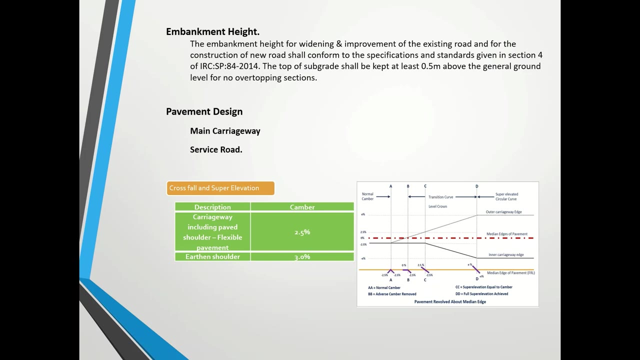 input or in open roads, whatever, you have to check the cross sections whether they are rotating properly or not. so that's why super elevation is a very, very important highway design element, okay. so because of that, only the means of drainage issues and whatever means vehicle can achieve the speed, okay. so that's why it is very important design element, okay. so next, 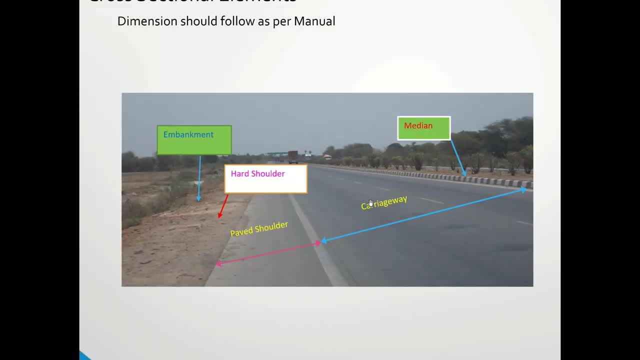 cross-sectional elements: see image cross section elements. so median carriageway and then pivot shoulder, hard heart, and shoulder means hard shoulder, nothing but embankment. okay. toe line: okay. so these values should be as per manual. okay. under tappers also should be as per manual, okay. 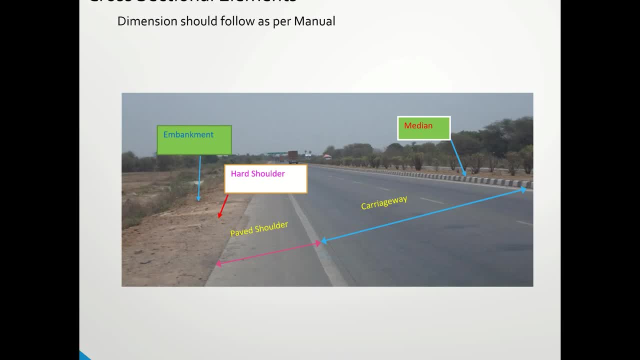 so try to means don't take independent decision. okay, yeah, you must follow the course, otherwise independent engineer will comment. so that's why the you have to follow the standards and prepare the line mode or whatever in templates according to the standards and standard cross sections provided and tappers also for median 1 in 50 and carriage 1 in 25 or 1 in 30. 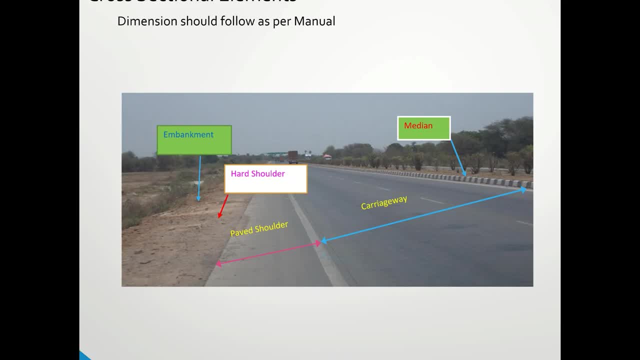 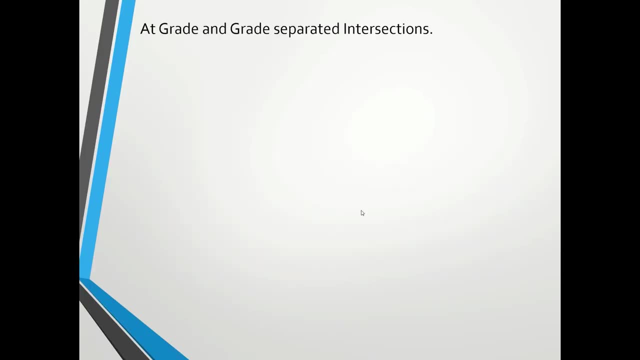 those things also you need to discuss with your manager. okay, then, only you have to take decisions. okay then, at grade and grade separated intersections, very, very important criteria, while using the vertical alignment vertical element, not only vertical alignment, because if you design the road itself, it won't satisfy everything, so you have to design the. 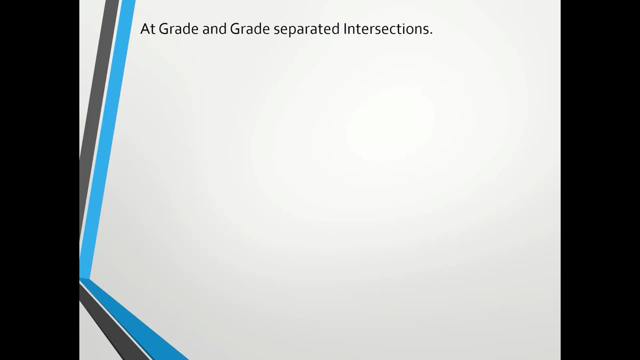 junctions, also to make maneuvers easily. okay, moment. okay, so there are ircs, special publication 41 and then irc 92. okay, grade, separated intersections, this and then major and minor junctions you have to identify. major junctions will be whatever the junctions uh creating with nh or sh or mdr? okay, some higher. 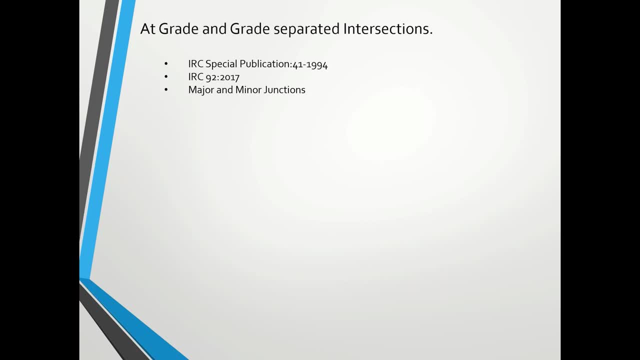 odr district. so if the width of the minor road is more than 7.5 meter, that also one criteria, but majorly type based on the type of road we use to decide whether it is major or minor junction. minor junctions will be for the village road zone, majorly based on the type of road we use to decide whether it is major or minor junction. minor junctions will be for the village road zone. 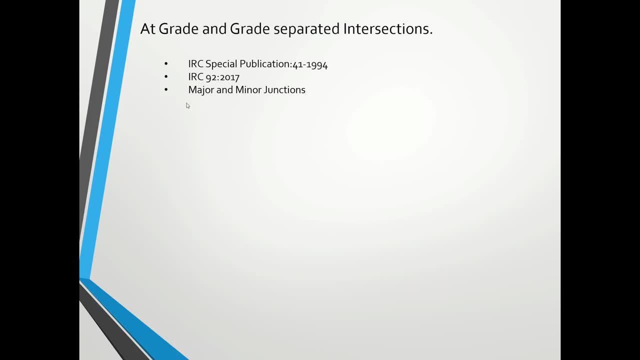 okay. so wherever major junctions are there, we need to provide the grade separated intersections. nothing but vups, cup or lvp. okay to move to, to make access controlled for the our highway design highway. so these are also important highway design elements. then, vehicle underpasses: what? 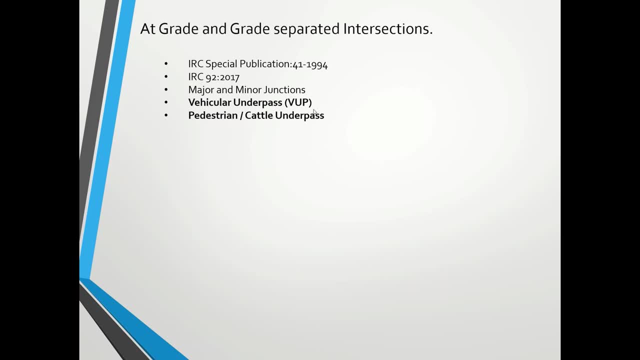 catalan purposes. while doing design of this, you must be aware about the clearance and frl values from the bridge department. okay, so from bridge department you have to take the finished road levels. okay, they will calculate it based on the type of structure. okay, so, whatever the clearance, 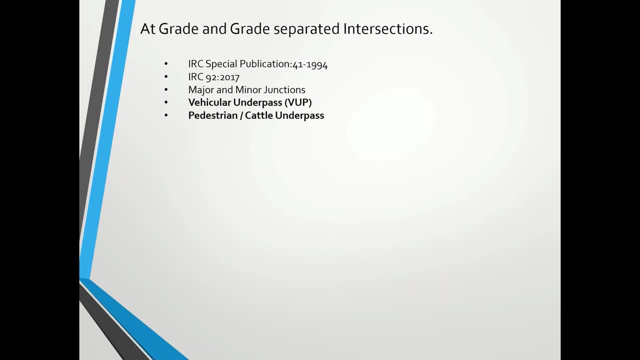 5.5 meter and the type of structure- if it is a gutter type, some 1.1 meter like that, so total around 6.6. okay, like that, and some camber correction- all things you have to evaluate and accordingly how to fix the frl okay. 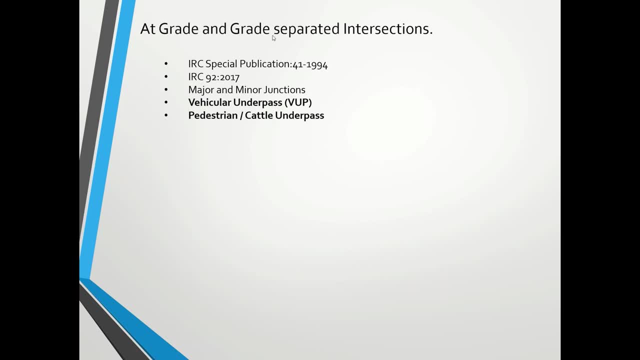 so fixing frl will be very important thing in grade separated intersections and normal grades junctions, mainly turning moment. okay, turning moment by either vehicle can move it or not. okay, so that can be you, that can. you can evaluate using the auto, turn software, whatever. okay, various softwares are there. okay, that can be vehicle path. also sweat path analysis. 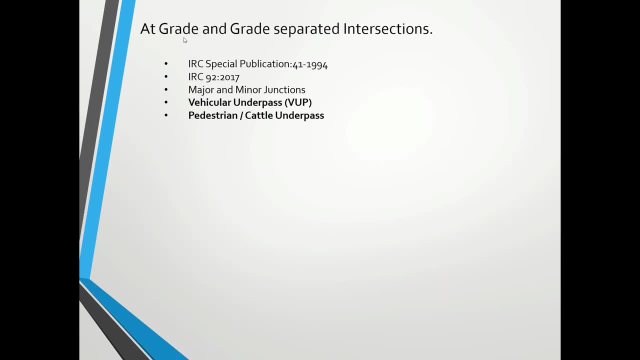 that also you can use while designing the at grade junctions. okay, some standard layouts are there. that also enough. okay, service roads, service roads, main thing: entry and exit ramps, okay, as per the ircsp 41, and then width should be 7 meter, 7.5 meter, like that. after that, service road profiles. 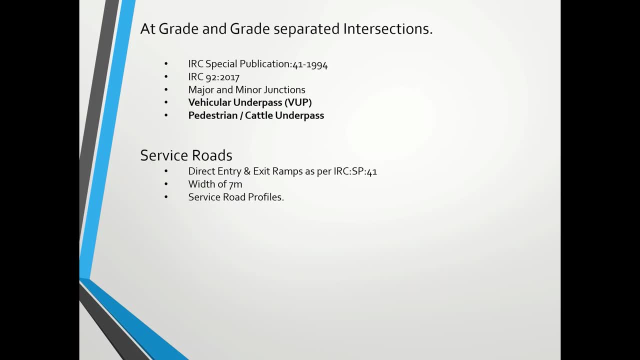 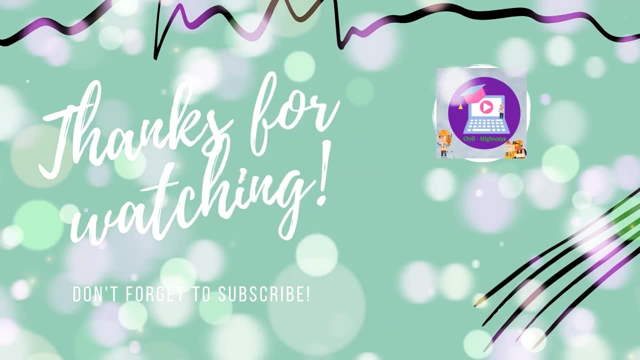 also very, very, very important, okay. so be aware, while doing the profiles. okay, if you want to fix your frl or you can use the frl part-time, you can use the front-end as well, okay, so let's go ahead and do a few more things, for the love of god. so we have the front end of the frl right here where this frl is, and then we have the back end of the frl- part-time. okay, that's great. we are going to bring that down a little bit here. bye-bye.